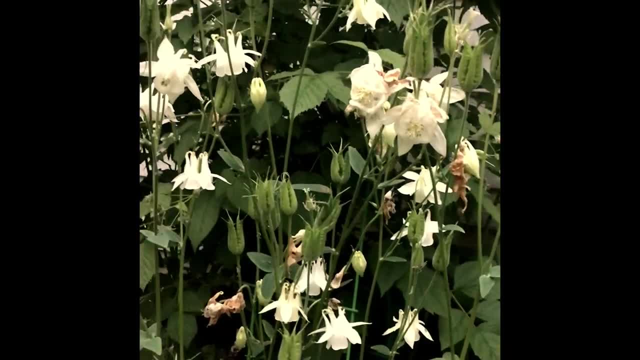 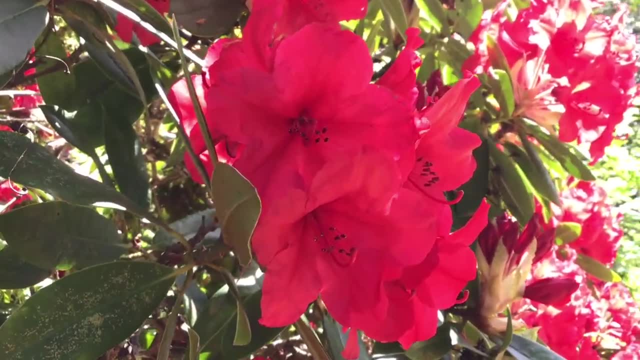 it is? Does it have a smell? You could name the flower, You could ask them what color or shape the flower, or talk about the different parts of it, like the petals, pollen or stamens, which exposes them to new vocabulary and concepts. 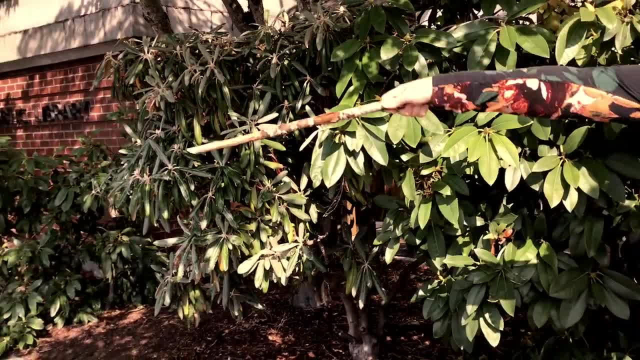 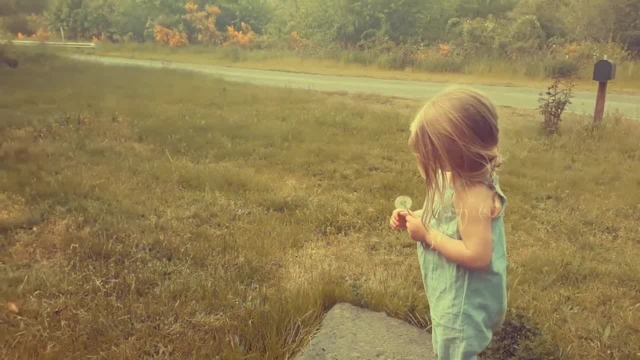 Another idea could be to make a magic wand with a stick or other things that you collect and have the children tell you stories from their imagination. This uses narrative or storytelling skills, which is another important component of early literacy, If you're working with letters. 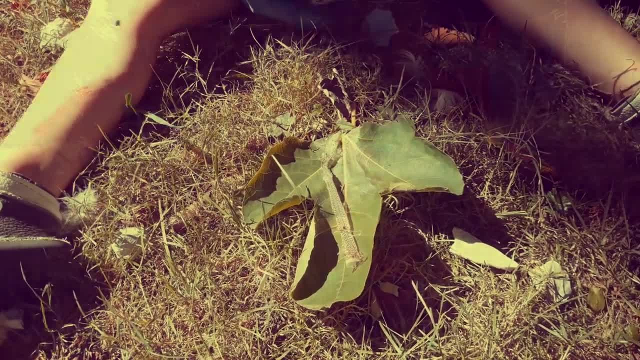 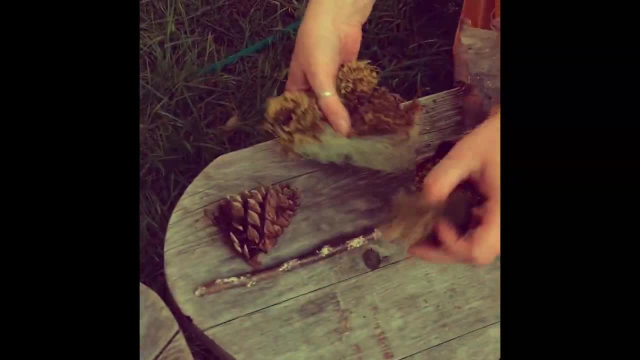 you could try to collect different things that start with a particular, like leaf for L or pinecone for P. Then explore the different materials you've collected when you get home. These items can be a jumping off point for a whole lot of other types of learning. 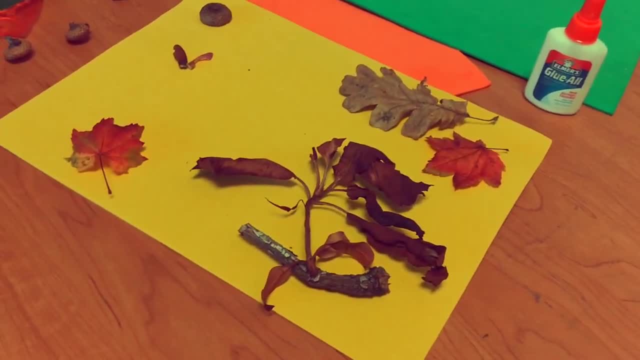 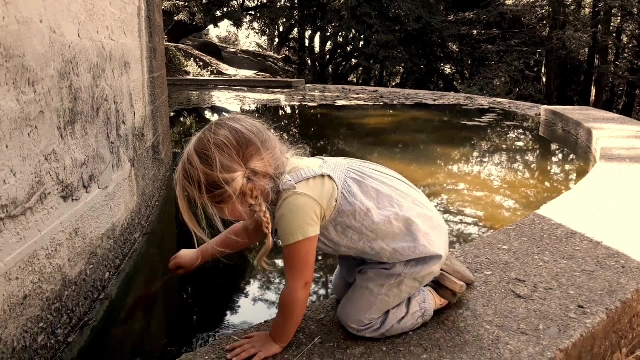 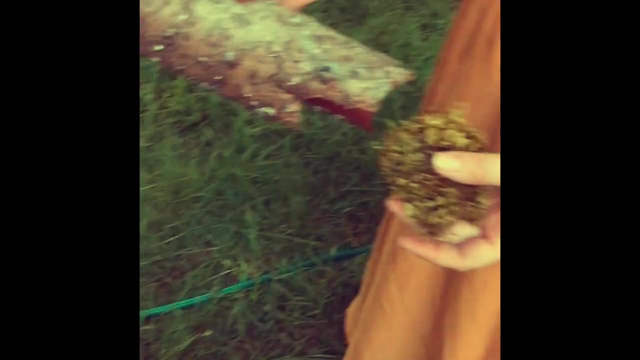 You could make a collage with the items, because research tells us that open-ended play offers important brain development opportunities for young children. You could see which items are heavier or lighter, or whether or not they sink or float. You could talk about the color or texture of an item, or even what are the materials themselves. 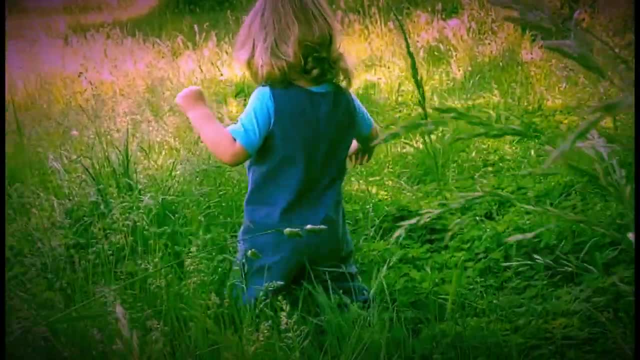 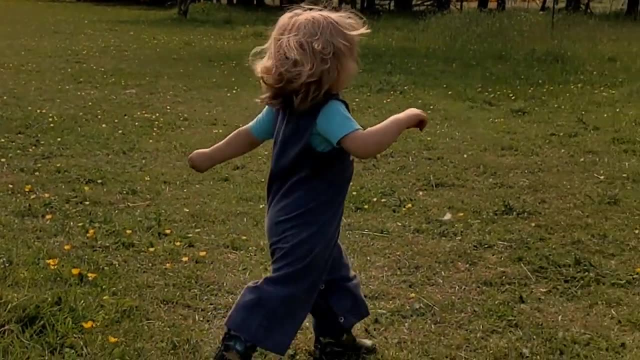 What purpose do they serve? What do they do? Children also learn a lot about earth sciences this way. By making the nature walk interactive, the things they've collected or seen will start to become interesting. They can now be used in all sorts of ways that build on the foundational skills. 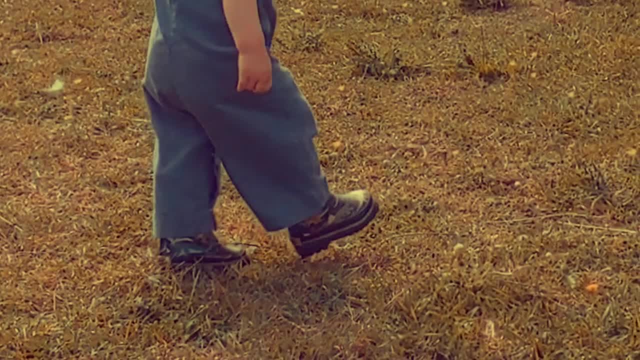 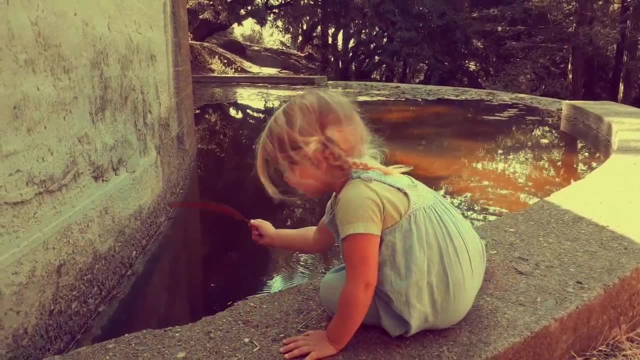 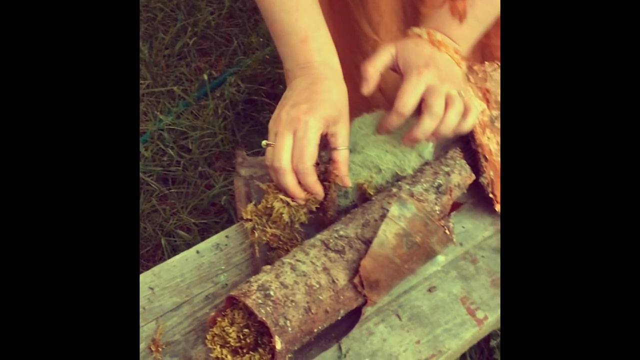 of literacy that go beyond the walk itself and can turn into activities that will spark imagination, creativity, play and learning, which are all critical to learning. A nature walk can also be an opportunity for children to learn how to respect nature. They're learning what things are natural materials, what are man-made. 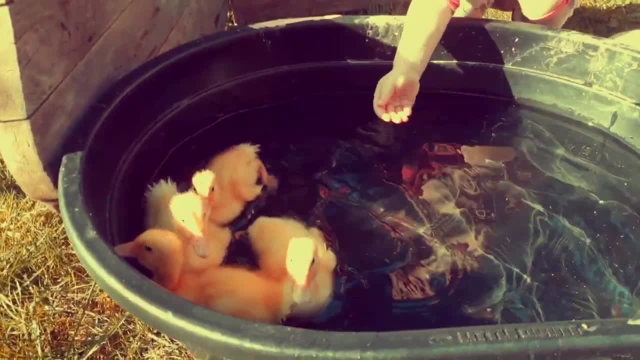 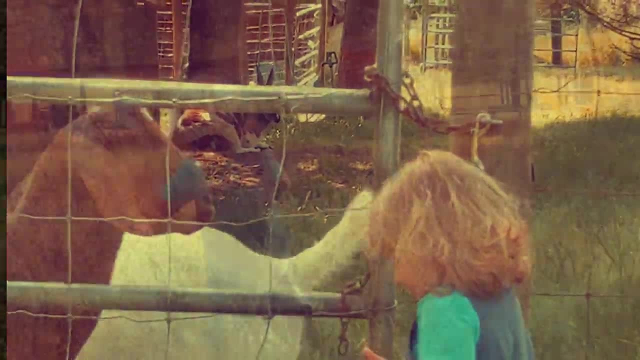 what kinds of things they can touch, what sorts of things they shouldn't touch. If you see an animal on your walk, you can talk about what the animal is, You can ask what sounds it makes. These things help with phonological awareness, which is an 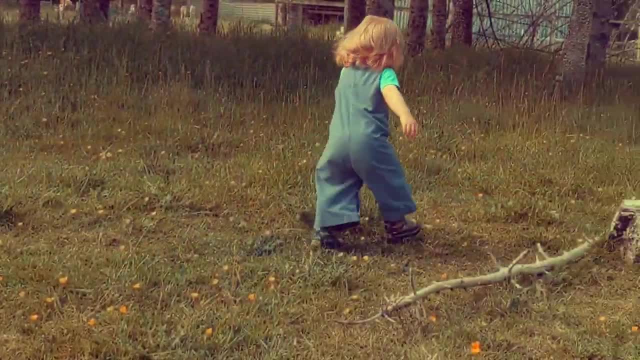 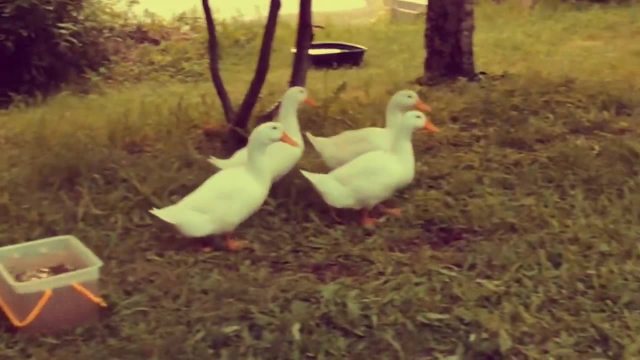 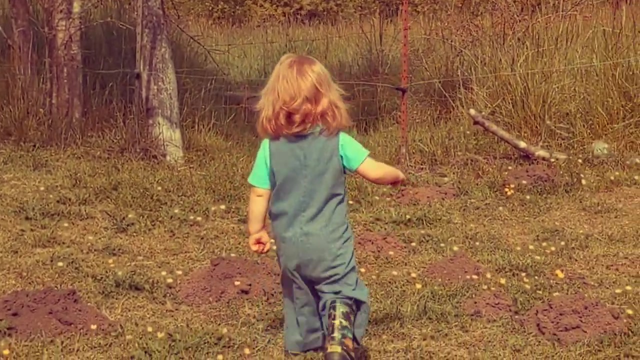 important skill that helps them understand, and growing the language, the subtle differences in words and sounds in language. This also provides an opportunity to learn about what animals are safe or unsafe to approach. Taking an intentional, interactive nature walk can have incredible benefits for children.